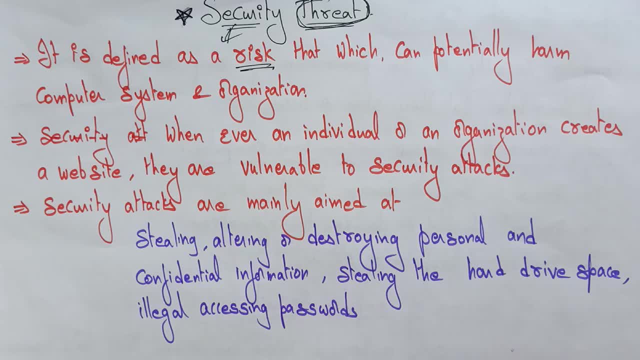 Okay, so we are working on the internet means we have to know about the threats that are occurring to your system also. Then you can aware of that. If you are aware of that, you can maintain your information safely. Okay, so in this concept, you are going to know what is a threat and what are the security threats. 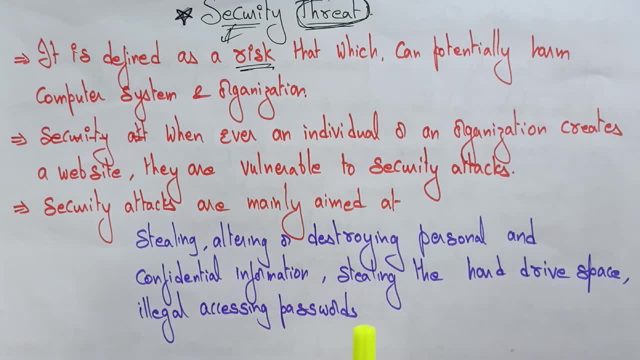 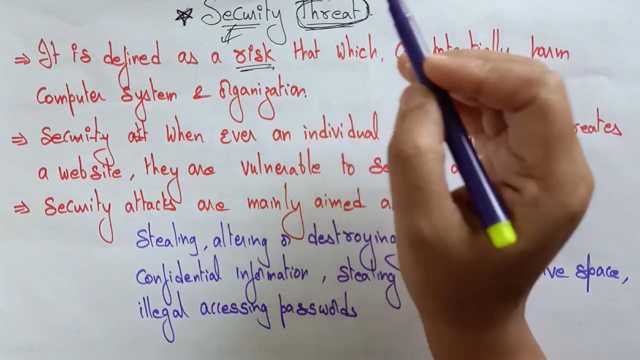 and what are the different types of threats that are means that are coming to your, means that are harming your system- okay, computer system, or even the organization, so that you are going to learn in this concept. okay, shall we start. come on, before going to know about the security threat, let's have 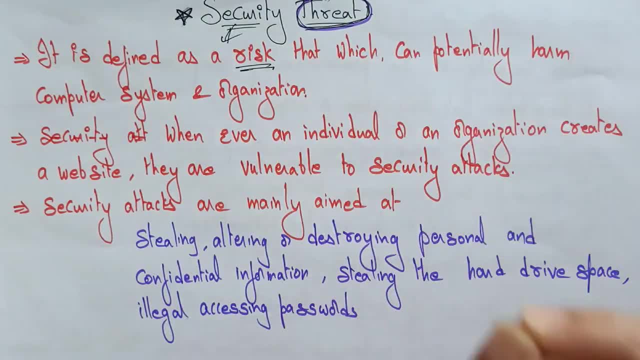 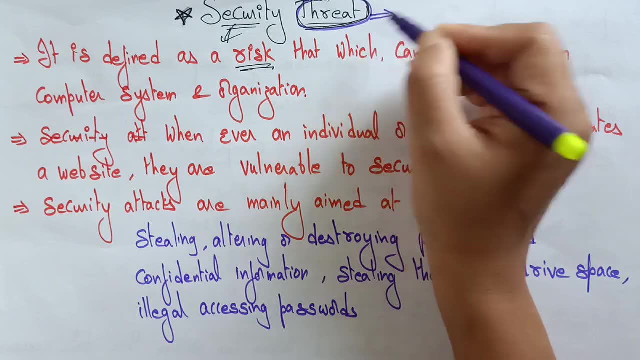 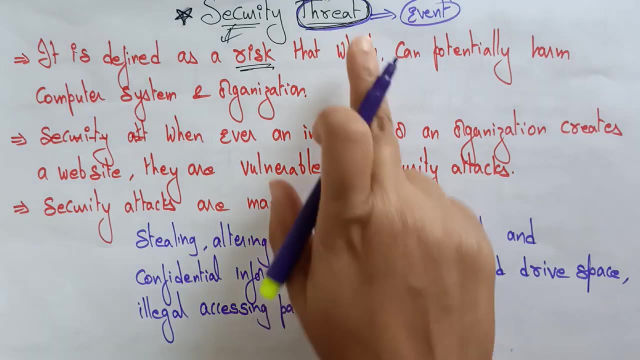 a look on the threat. what is a threat? a threat is nothing, but it is a possible event that can damage or harm an information system. so a threat is nothing, but it's just simply an event. a possible event means a simple code that is going to damage your system. that is a threat. then what is a 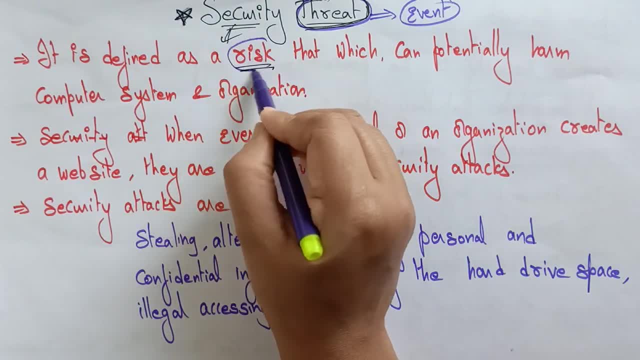 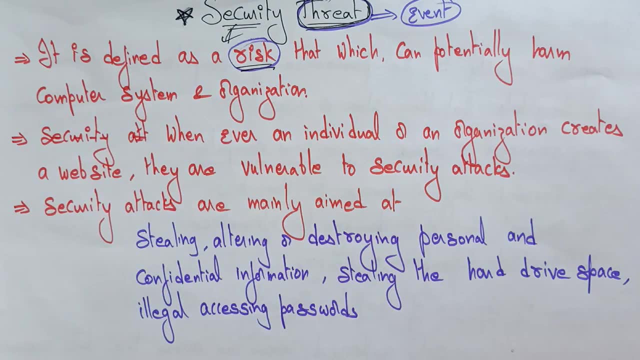 security threat. security threat is defined as a risk, that which can potentially harm a computer system and organization, that you call it as a security threat. whenever an individual or an organization creates a website, they are venerable to security threats. so obviously suppose, if you are having an individual system, let's take your. 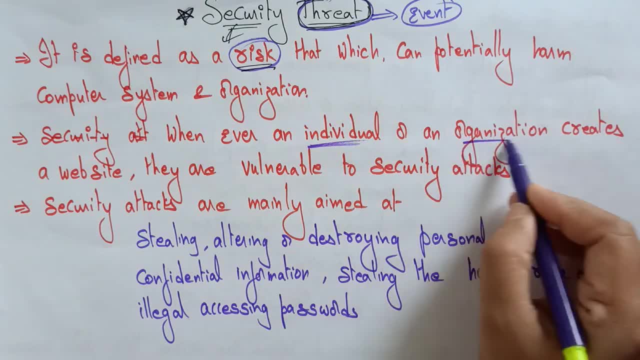 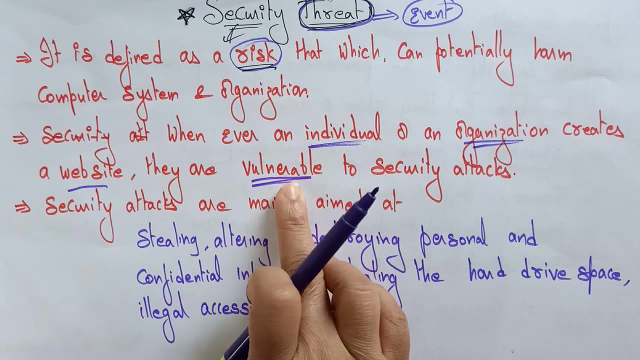 system. or if you are working on an organization, so take the organization. so here the individual or organization. suppose they are going to create a website, let's, let's. they are going to create a mini website. they are venerable to security attack. so what is this venerable? venerable is. 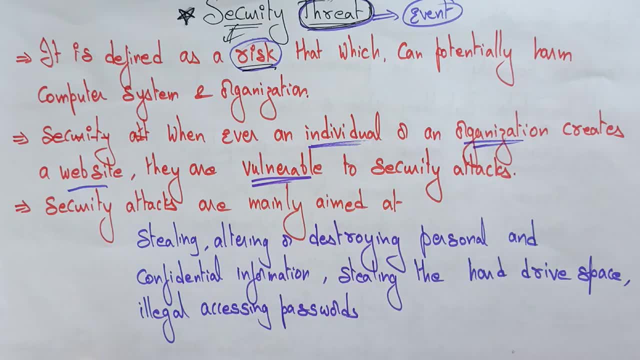 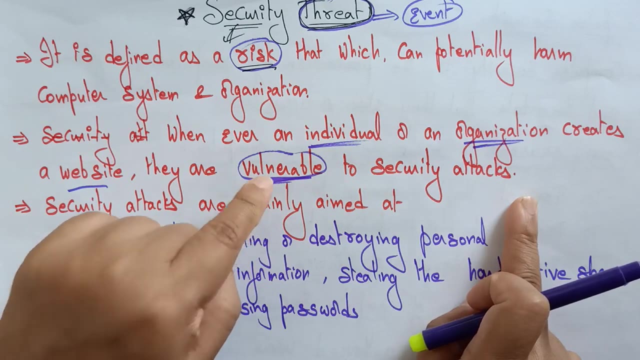 nothing, but it is a weakness within a system. so it is a degree of exposure to view of a threat. so it is, whatever the website that you are creating, they are venerable. that is, it is a weakness within a system to security attacks. because of this weakness, because of this venerability, our system, 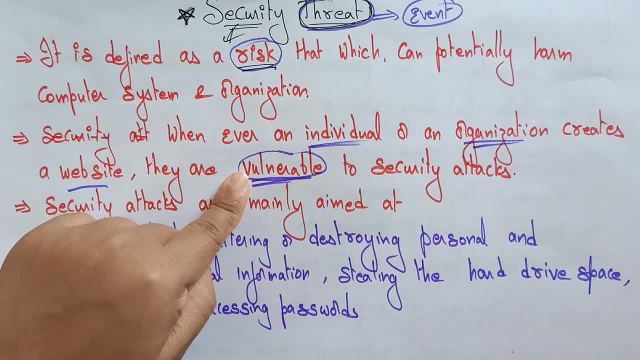 is going to attack a security attacks are going to be applied on your website, so the security attacks are mainly aimed at. so what they are going to do, what this security attacks on your website or in your application. so, whatever it may be, so whatever the website that you are creating, 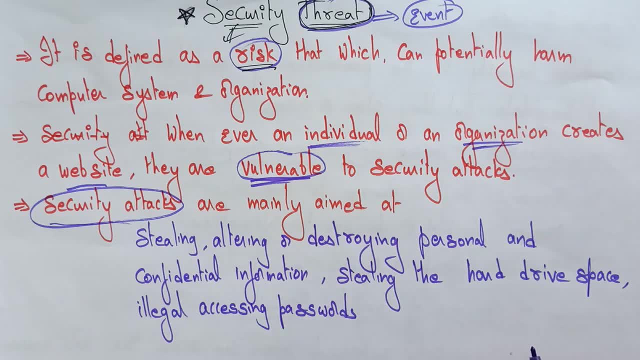 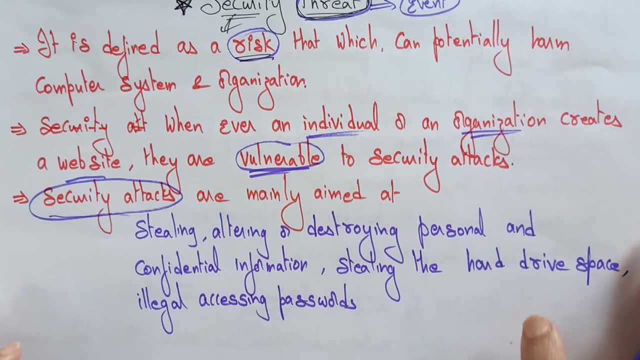 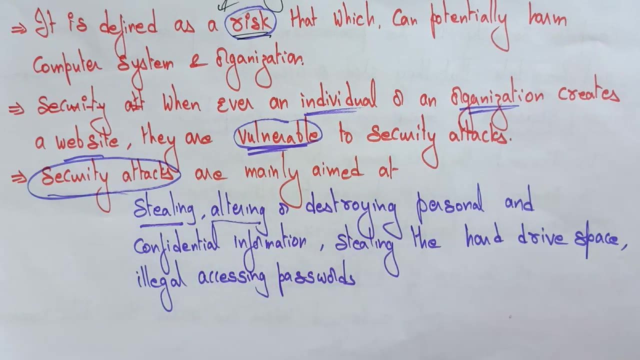 this is a simply an event of a simple code which is going to install in a computer. so what it is going to do, so what these attacks are mainly aimed at. so these security attacks are mainly aimed at stealing. stealing means acquiring, altering, changing or destroying, even though it is destroying the 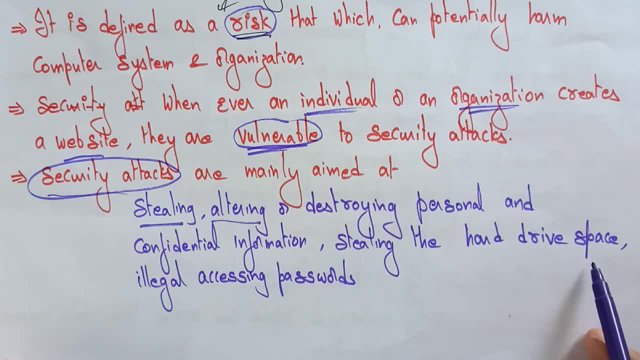 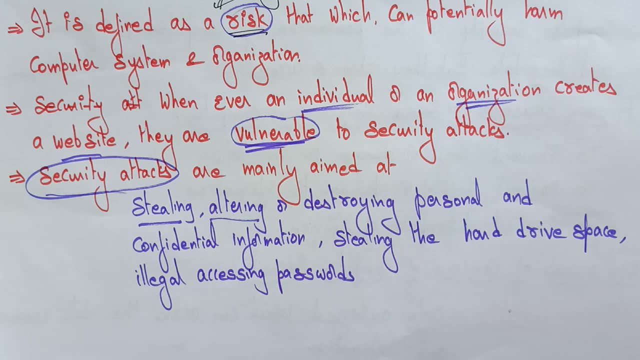 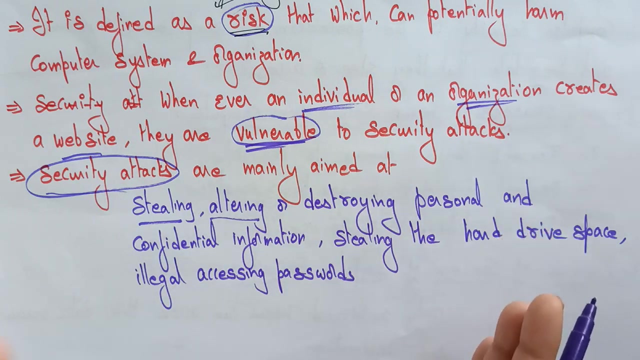 personal and confidential information, stealing the hard drive space, illegal accessing passwords. so these are all the things that these security attacks are going to do in your system. okay, so when the security attacks are going to stay means, or focusing on these things, whenever your website, whatever you are created, they are venerable to security attacks, then your security attacks are. 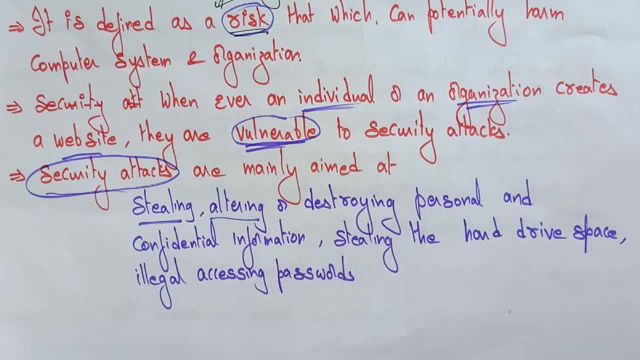 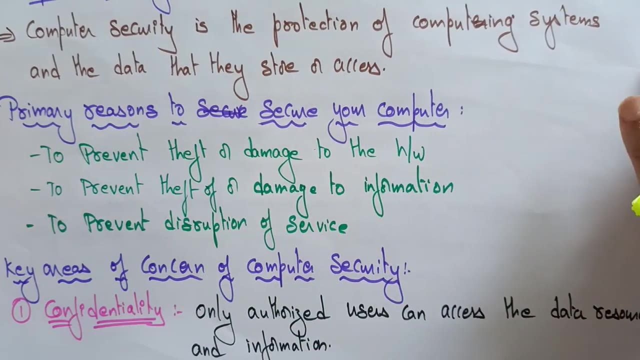 going to steal your data, alter your data or destroying your personal information, and it's seeing your confidential information and also it accessing your passwords also. so the security attacks aims, or this, okay, a computer security, uh, basic. so what exactly the computer security bit let's talk about? uh, a system, a computer system. 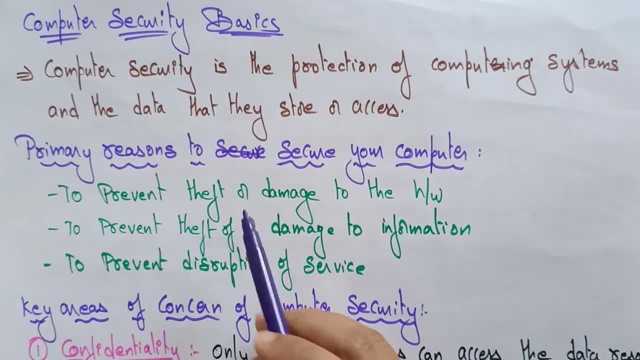 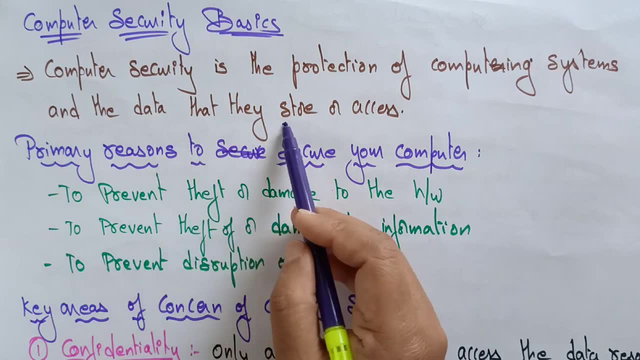 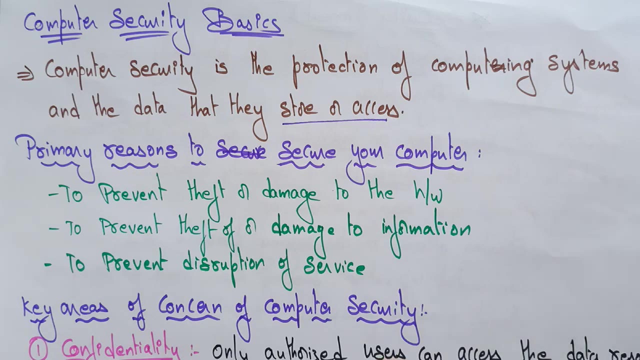 so what a computer security basics will be? a computer security is a protection of a computing system and the data that they store or access. let's take your personal system. so if you want to have a computer security, uh, so what it is going to do if we are just providing a protection to your? 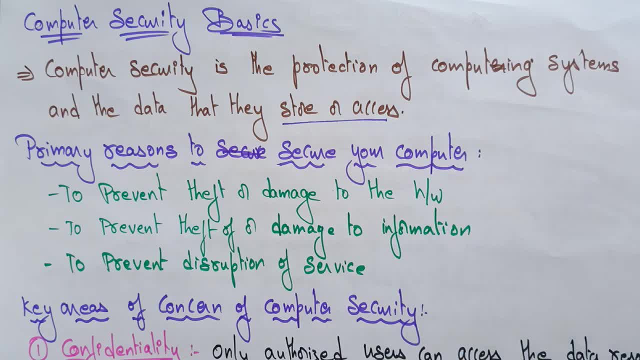 computing system. and also we are providing some protection to our, to your data which stores or access- okay, the data that they store or access. so we are providing some protection to that data which is going to store our access, so that you call it as a computer security. 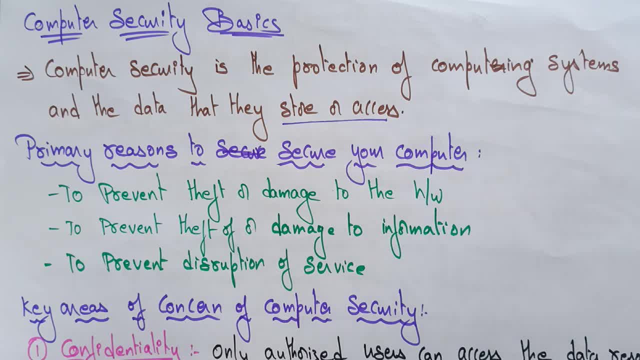 so what is the primary reason to secure your computer? so why we are, uh, you're all going in your system. you are going to install your security, okay, some softwares you're going to uh install. so actually, why? what is the primary reason to secure your computer? is it very uh required means it is. 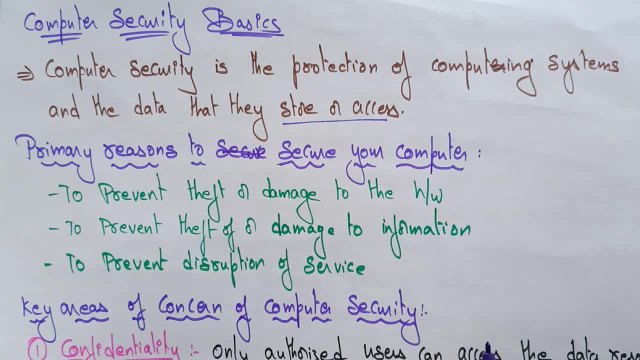 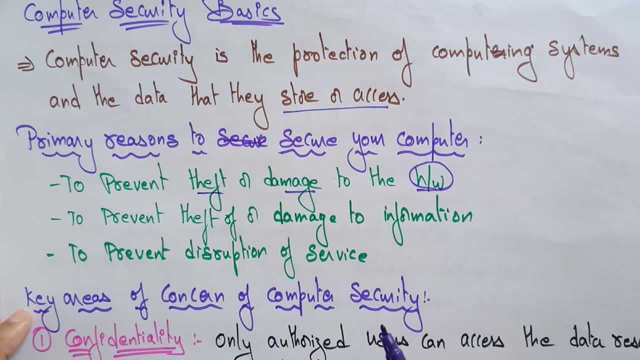 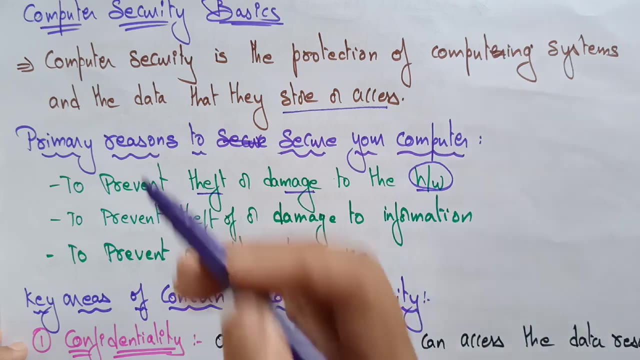 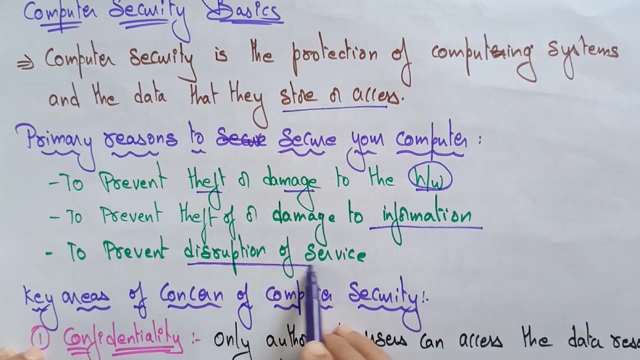 important that you need to secure your computer. obviously why? because to prevent the theft or a damage to the hardware. so if some attacks or occur, the security attacks or occurred in your system, it is going to damage your hardware. so to prevent that we are using the security. so to prevent the theft or a damage to information also and to prevent the disruption. 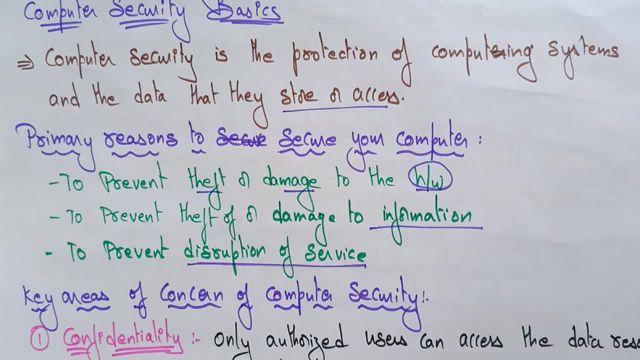 of a service, even your service, means when you are working on something, some because of the security attacks, your services will be disrupted. okay, like if you are doing some online shopping or some you are doing some online activities, so these attacks security act attacks or disrupt your service. so because if you install the computer security software, it is prevents the. 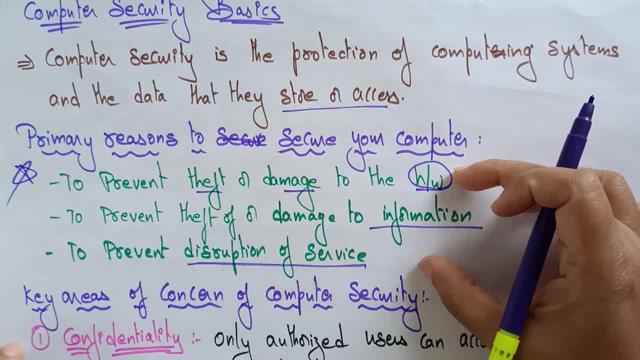 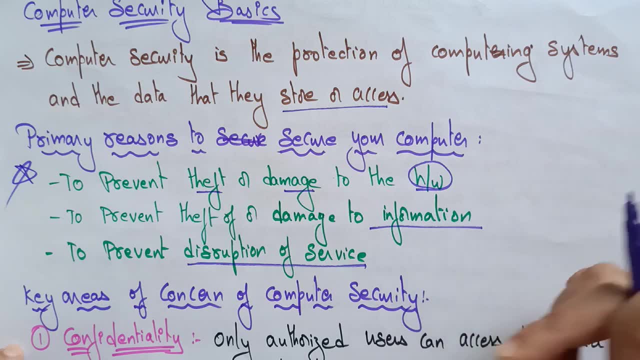 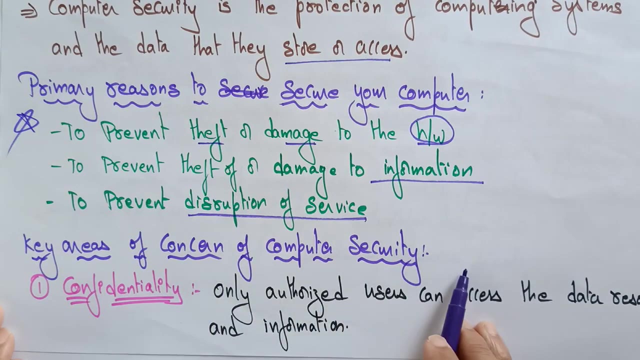 disruption of the service. so that is a primary reason to secure your computer: a prevent or a theft on hardware to the hardware and to the information, and to prevent the disruption of services. now let's have a look on the key areas of concern of computer security. so the key areas: 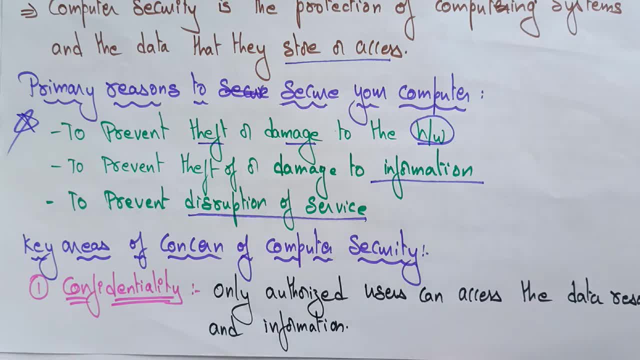 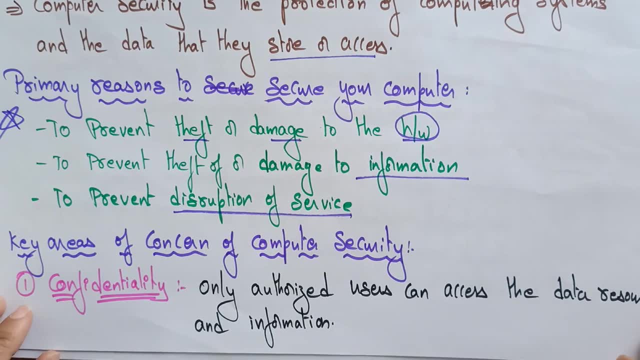 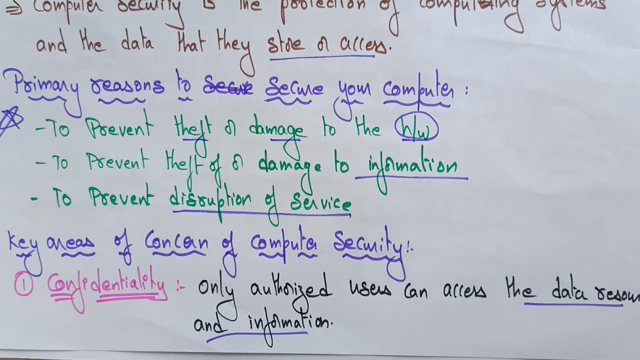 of concern of computer security is: first thing is the confidentiality. confidentiality, that means only the authorized person- user- can access the data, resources and information. that is the meaning of the confidentiality. so what is computer security will doing on your system? it is just maintaining a confidentiality. so what is this confidentiality? 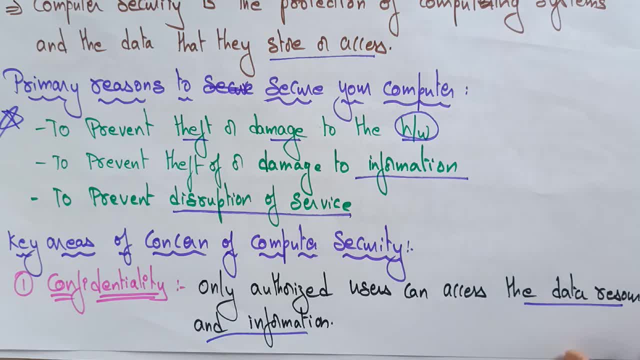 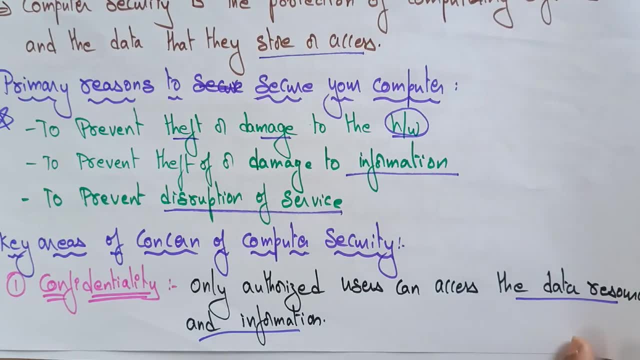 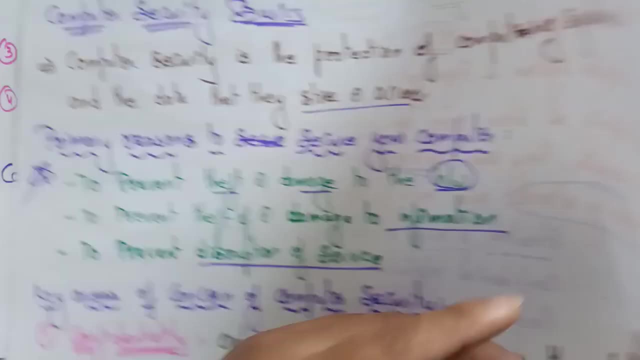 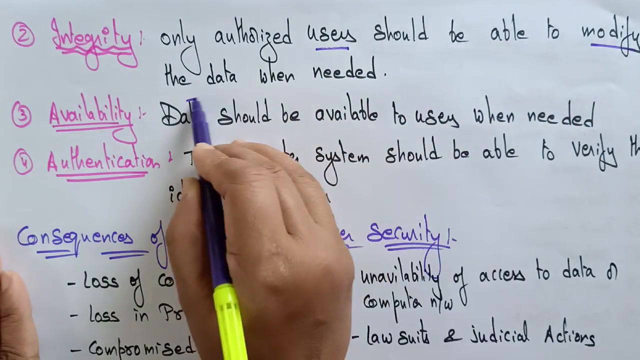 only the authorized person means suppose you are, if you are given some username and the password, only that person can access the data, resources and information. other than that no one can access that information. so you can maintain confidentiality if you concern on the computer security. next is integrity. integrity means only the authorized user should be able to modify the 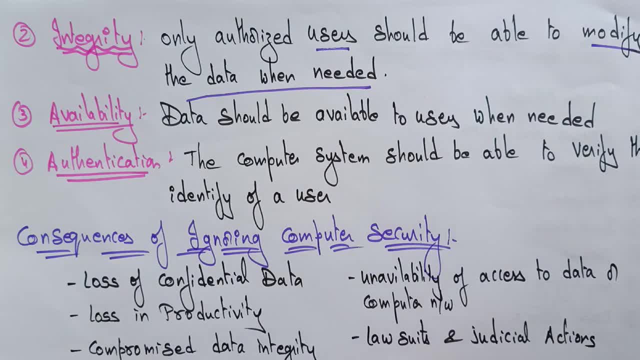 data when needed. so suppose, if you want to change some information, or if you want to override some information, or if you want to delete some information, so like that, so only the authorized user can do this work. okay, that is the integrity. so it is maintaining the confidentiality and integrity availability- availability means only the authorized person. 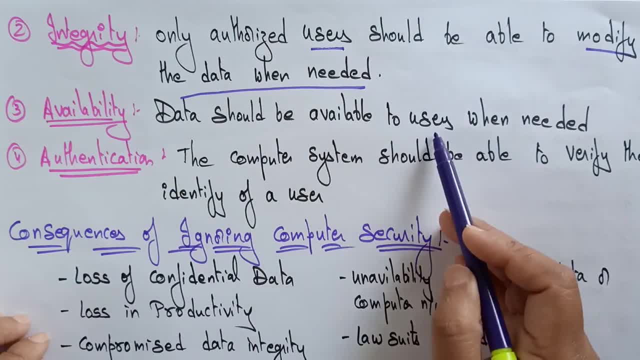 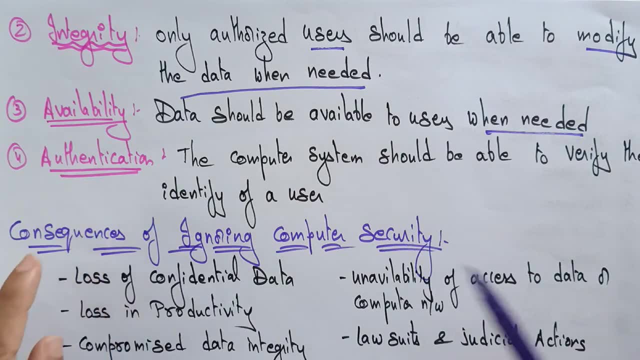 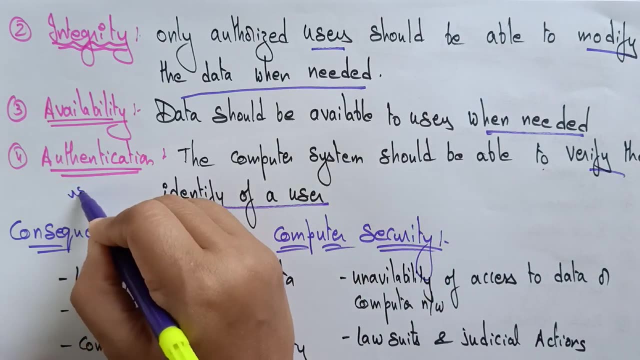 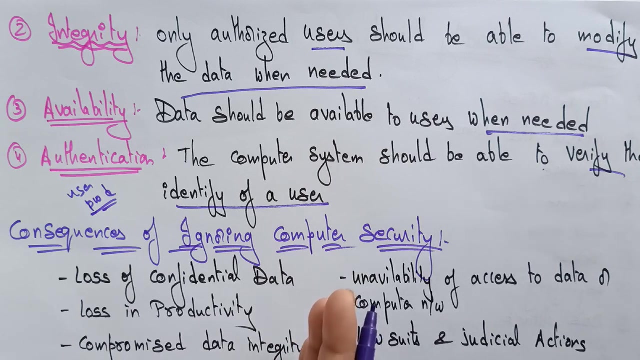 can able to see the data. data should be available to the users when needed, whenever it is needed. only the authorized person can see that. and authentication? authentication means the computer system should be able to verify the identify identity of a user, like this username password. okay, so that is authentication. so these are the key areas of concern of the computer security. the 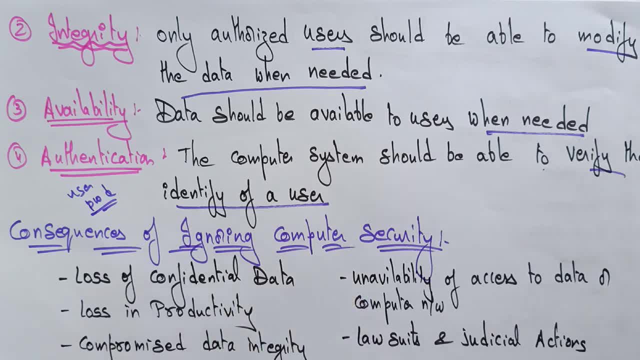 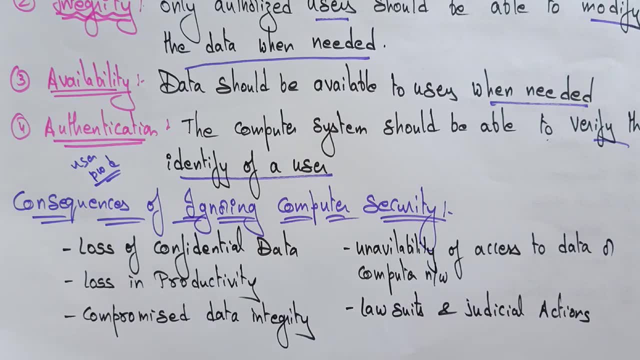 computer security is focusing on the confidentiality, integrity, availability and authentication. okay, so next, suppose, suppose, let's take: uh, i don't want to concentrate on those things. i don't want to concentrate, that means i don't want to install the computer security to my system. then what will? 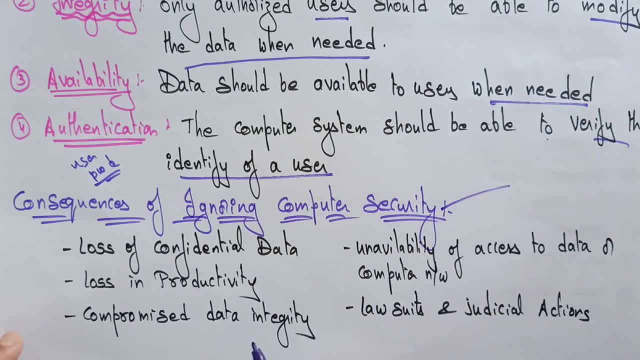 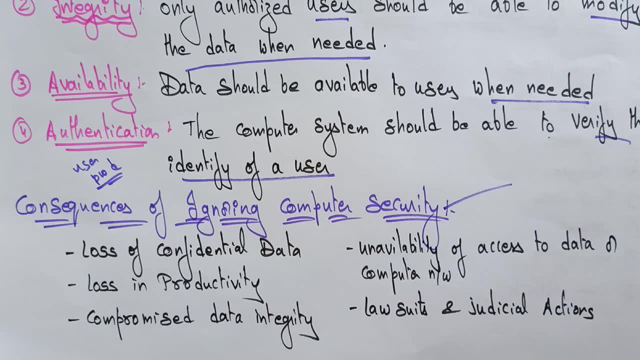 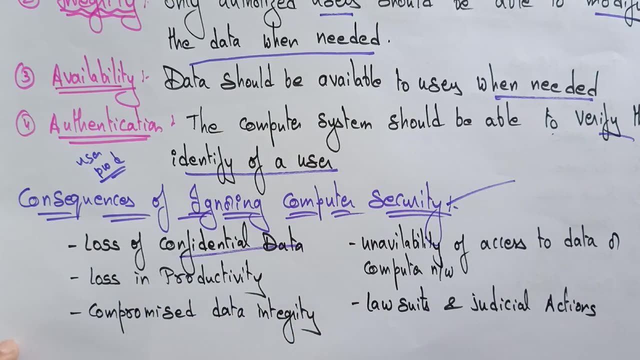 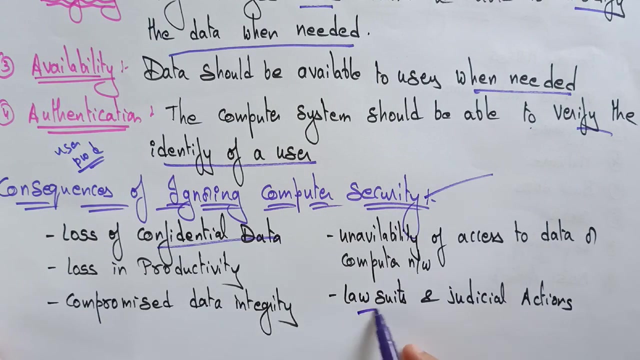 happen? the consequence of ignoring the computer security? suppose if you didn't install any the uh software like the security software, okay. so what will be the consequences if you ignore that? the loss of confidential data, loss in productivity, compromised data integrity, unavailability of access to data or computer network, lawsuits and judicial actions. so these 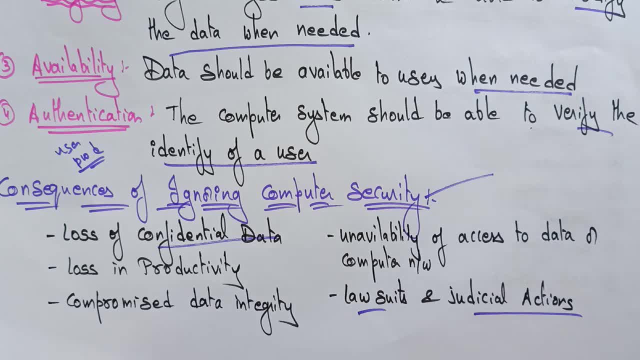 are all the consequences if you ignore the computer security. so try to maintain a computer security so that your data cannot be damaged, your hardware cannot be damaged and your information cannot be theft. okay, and there should not be any disruption of the services. so what this computer security is going to do, it is going to maintain the confidentiality, integrity, availability and 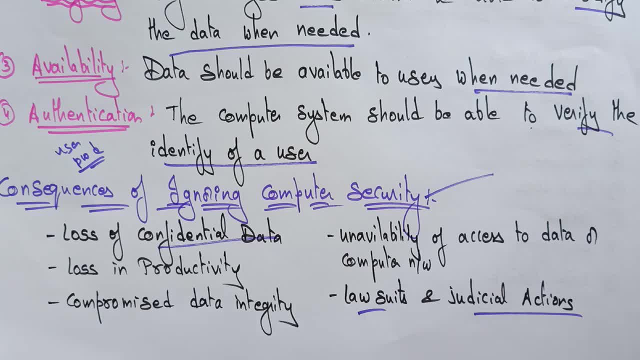 authentication. so this is a simple introduction part of the security threats, okay. so what i explained, what is a security threat- okay, and what i explained: okay, what is the main aim of the security threat and what is the primary reason to secure your computer and what are the key. 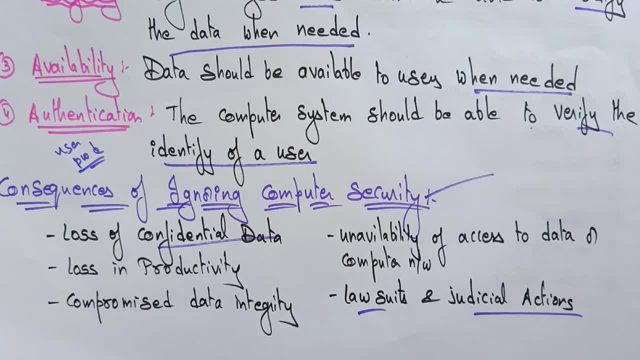 key areas of concern of computer security. so this is what i had explained in this video. so it's just a basic introduction part of the security thread and the next video we will see about the different types of the security threads. okay, thank you.